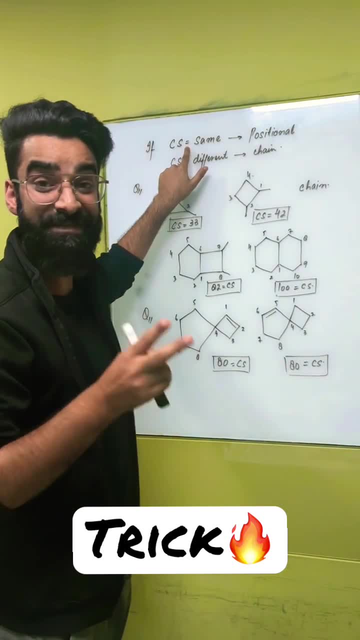 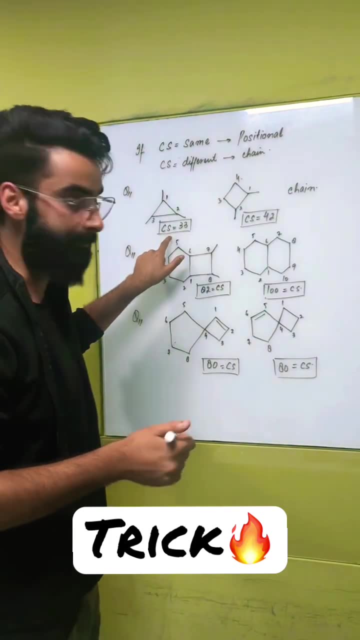 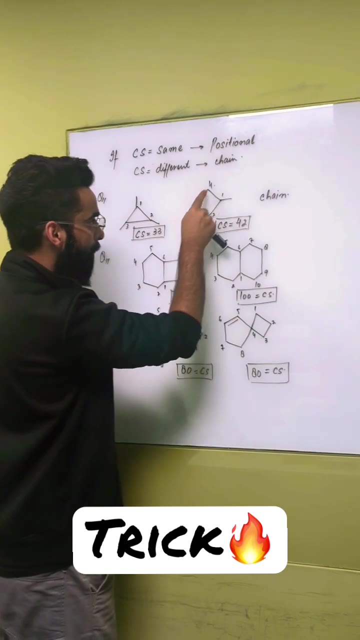 substituents starting with carbon For two isomers. if CS value comes out, be same positional. If CS value comes out, be different chain. Look at this particular equation. In the main chain you have about three carbon atoms. There are three substituents starting with carbon. So CS value is 33.. Main chain: four carbon atoms. 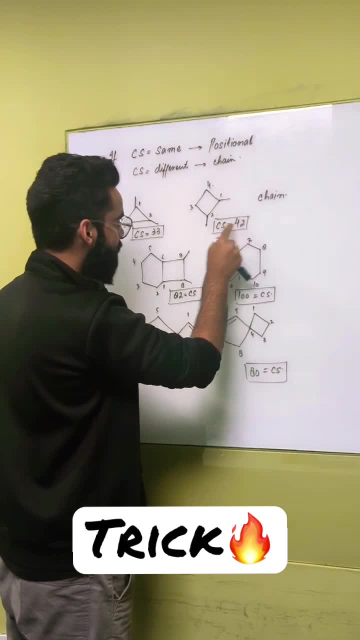 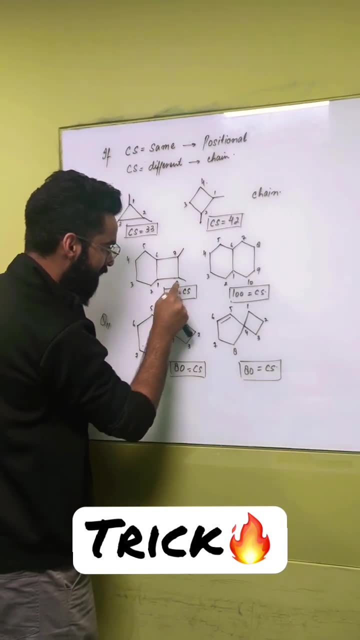 Two substituents starting with carbon, So 42.. CS value comes out be different, So chain isomers. Similarly, in the main chain there are eight carbon atoms Right, So C value is eight. Two substituents starting with carbon, So 82.. Similarly in 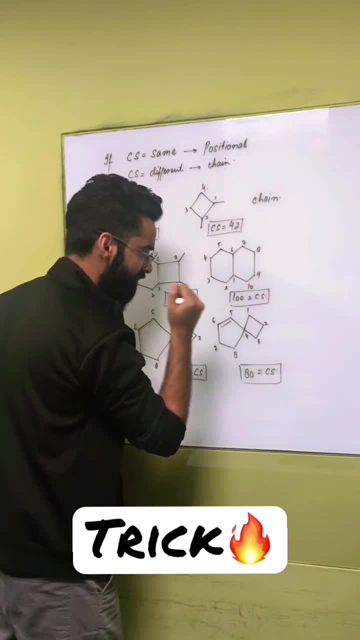 the main chain, ten carbon atoms, No substituents starting with carbon. So CS value is 100.. Since CS value is different, I mean chain isomers. Let me know the answer of this particular question in the comment section. 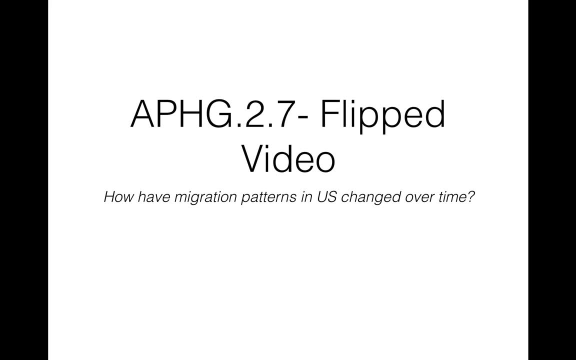 We're going to continue our discussion of migration with our next essential question for 2.7 of how have migration patterns in the US changed over time? So we're going to be looking at the origins of the people coming to the United States. We're also going to be looking at some of the internal migration in the United States. 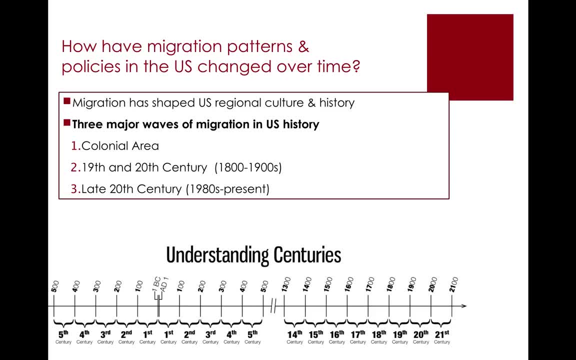 So migration in general, the reason why we talk about this relative to the US is in AP we are looking a lot at how the migration patterns, the historical migration patterns, help explain the cultural and regional differences in the United States, because it really has. many of those differences have their heart and their core in who came and when they came and why they came. 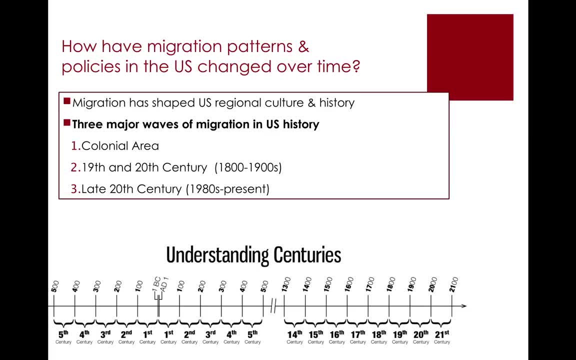 So, in general, there are three major waves of migration in US history. according to AP Human Geography, Our first is going to be considered the colonial era, The second will be the 1930s, The third is the 19th and 20th century.